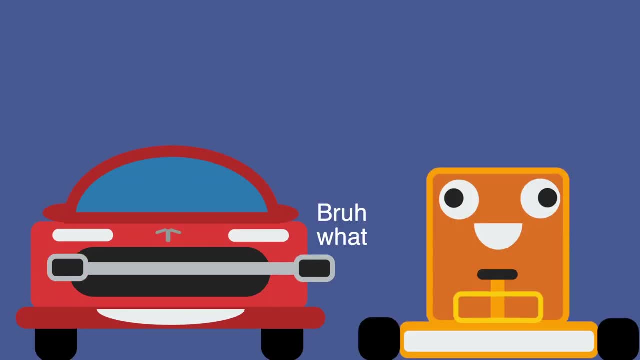 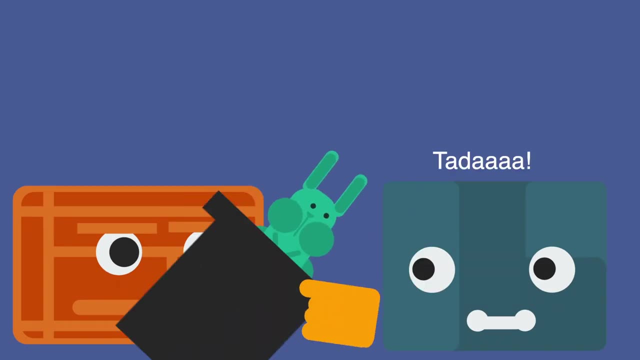 equivalent of Elon Musk unveiling the next Tesla model to be a go-kart. The computation used to prove quantum supremacy would be a cheap parlor trick. In fact, the earliest quantum algorithms from the 1990s were just that cheap parlor tricks. Do I care about identifying whether or 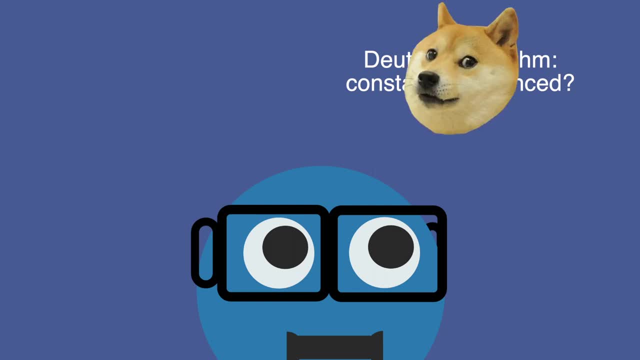 not. a function is constant or balanced- Absolutely not. Does the fact that a function is 1 to 1 or 2 to 1 impact me in any way? Not at all. Does a quantum computer's ability to find the prime factors of any number have any relevance in my life? 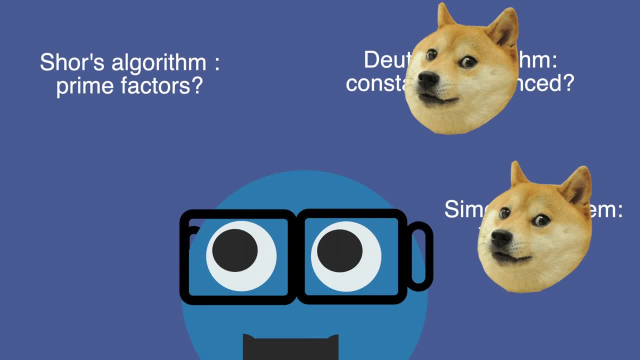 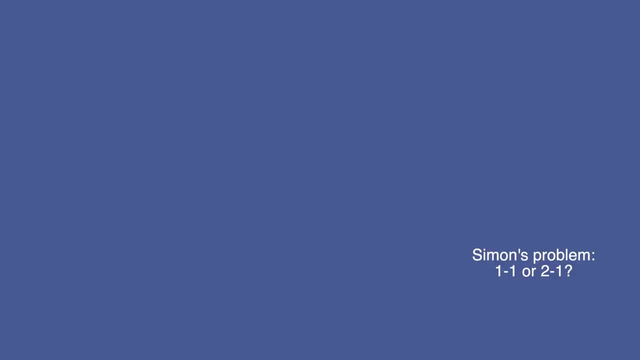 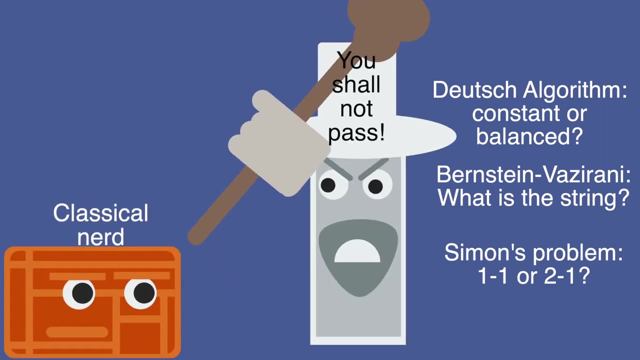 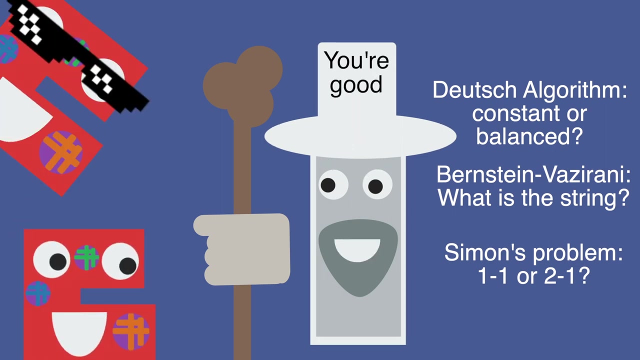 Actually this one does, because it could render RSA cryptography useless and nullify all privacy on the internet. The aforementioned algorithms are important because they demonstrate that there are indeed problems that only a quantum computer can effectively solve. Those were the necessary predecessors to the more practical algorithms that get the spotlight nowadays, such as Grover's algorithm. 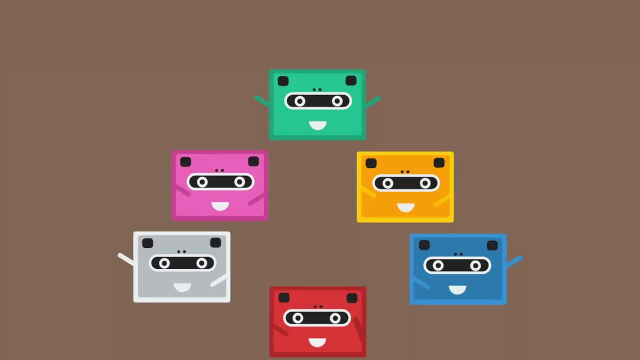 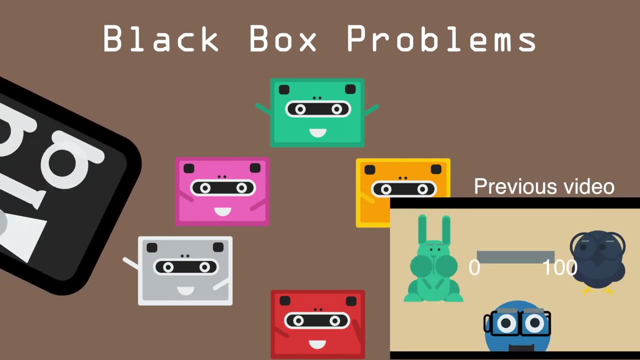 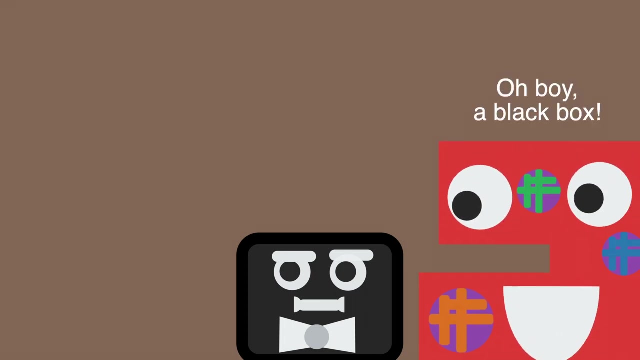 and Shor's algorithm. These ancient quantum algorithms are collectively referred to as the black box problems. Huh, black box. you say How convenient. We just spent 4 minutes and 11 seconds discussing black boxes. What are the odds? The reason: a black box is the perfect platform for constructing quantum. 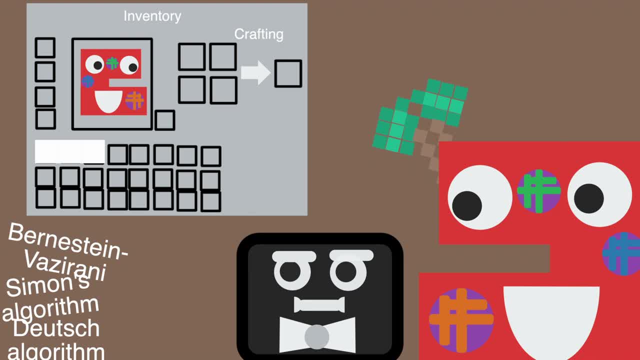 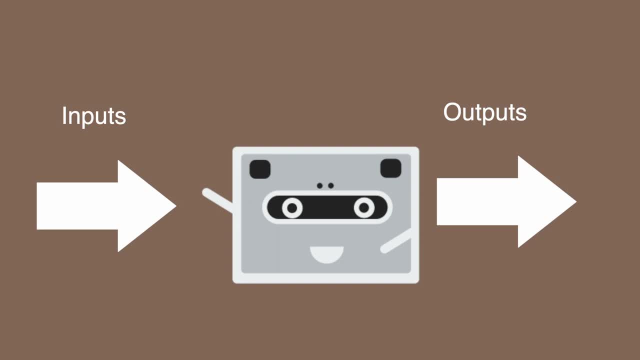 algorithms is because of its generality. In the last video we saw that the only relevant components of a black box are the inputs and the outputs. The only information my friends needed to discover my number was a numerical guess and the higher or lower response. I provided Nothing about the properties of 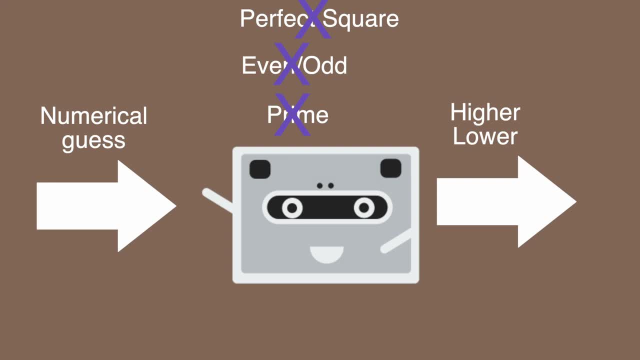 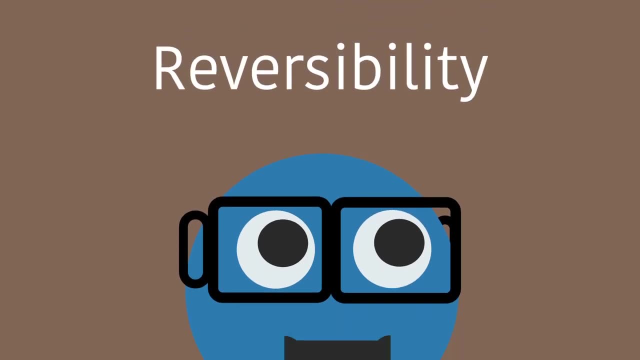 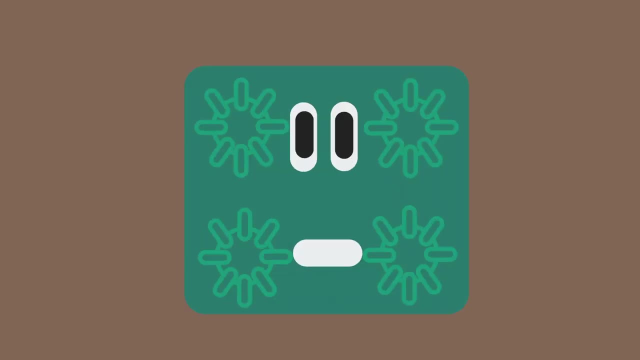 the number, ie the internal design of the black box was necessary, But before we continue, we must discuss an essential concept in quantum computing: all operations must be reversible. What is reversibility, you ask? Here is an operation that accepts two inputs, either of which can be a zero or 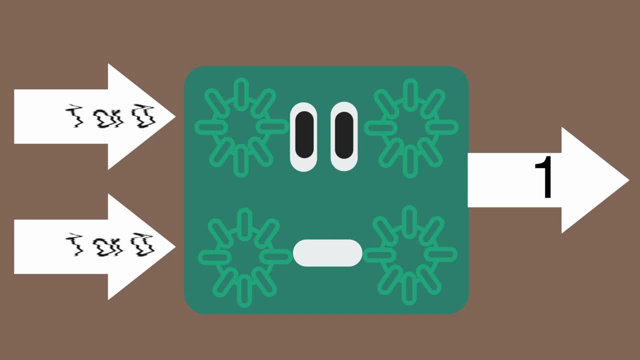 a one. It will output a 1 only if both inputs are 1.. If I hide the inputs and you see an output of 1,, you know for a fact that both inputs were 1.. However, if I hide the inputs and you see an output of 0,. 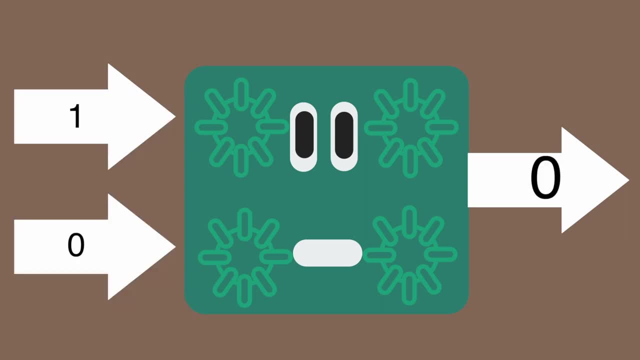 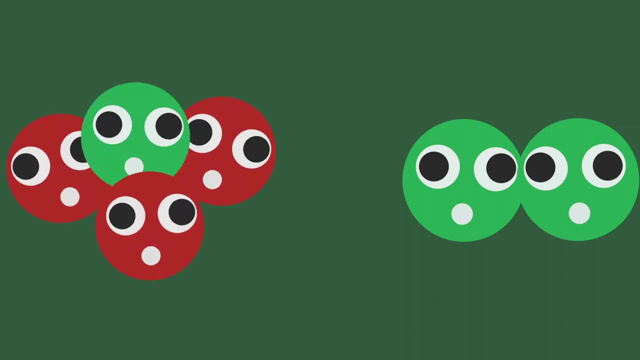 you don't know whether the inputs were 0 and 1,, 1 and 0, or 0 and 0. In other words, information was lost. Since there are two possible outputs and four possible input combinations, it's impossible for this operation to be reversible. 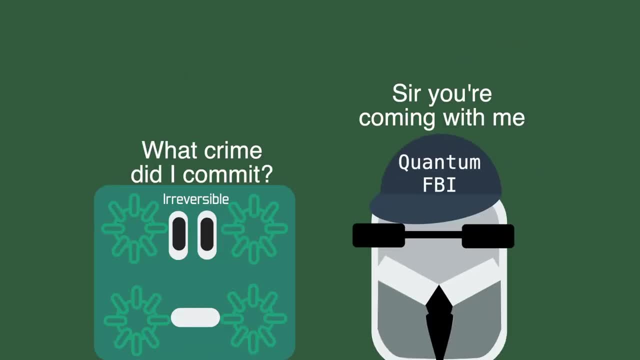 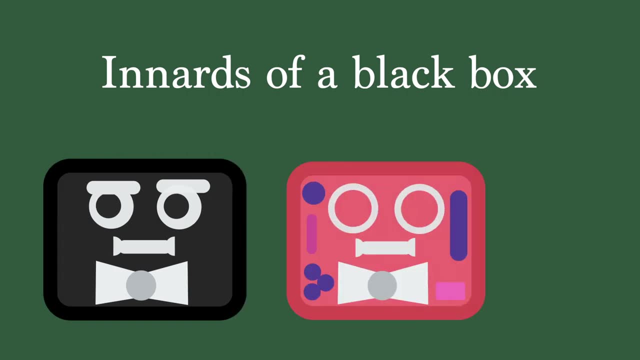 Quantum computing forbids this. We must be able to rewind an operation and acquire the inputs just as easily as we obtain the outputs. And since quantum black boxes consist of quantum operations, even if we don't know the details of those operations, the black box must be reversible. 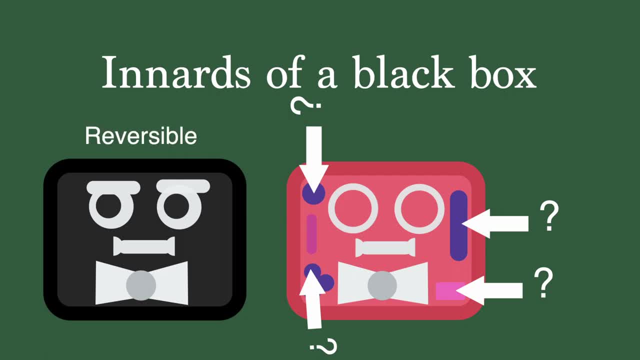 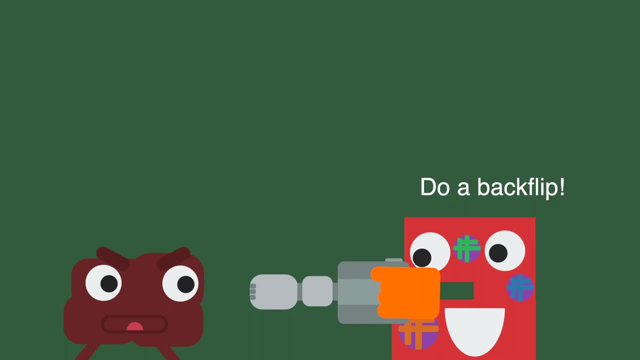 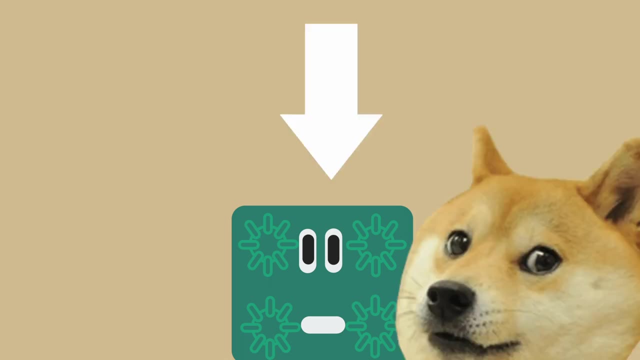 Therefore, the number of inputs and outputs must be equivalent. Quantum oracles are mathematically adjusted to accommodate this requirement. Okay, now that we've established the basic rules, let's see this all in action. The black box problem. The black box problem is a very common problem that is often referred to as the oracle. 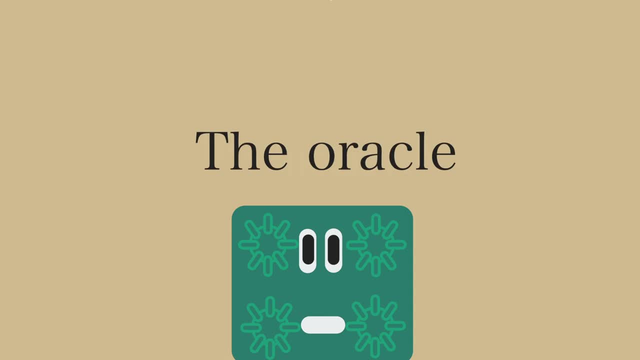 The oracle performs some function f on some number of inputs consisting of 0s and 1s and produces an equivalent number of outputs consisting of 0s and 1s. Our goal is to determine some property of this function. The Deutsch problem is a good demonstration of this. 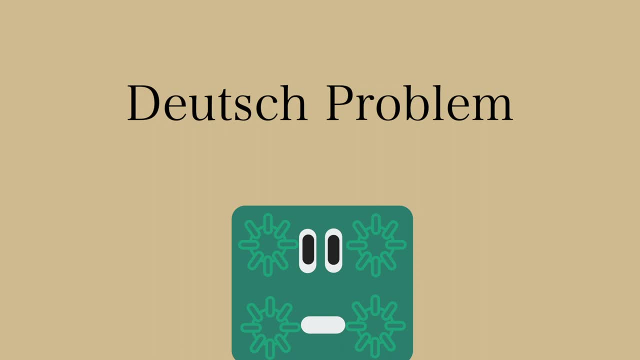 This oracle can produce two types of outputs: A constant output, which outputs 0 regardless of the input, and a constant output which outputs 0 regardless of the input, Or a balanced output, which outputs an equivalent number of 0s and 1s. 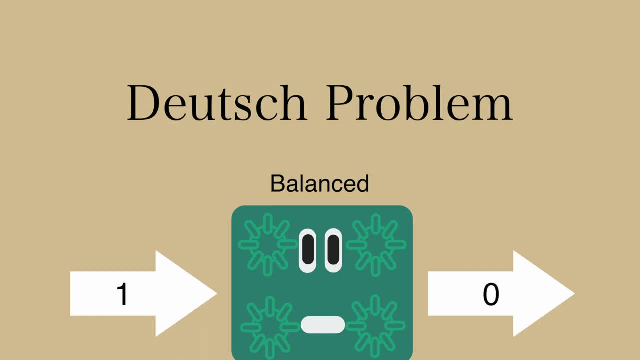 The problem is to determine whether the oracle's function is constant or balanced. A classical computer would need to ask the oracle to perform the operation twice to answer this question, because it needs to know what happens to a 1 and a 0 separately. 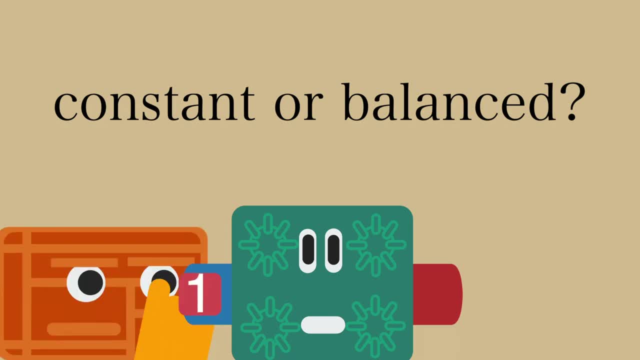 and then compare those results to see if they were the same or the opposite. The Deutsch algorithm proves that a quantum oracle can produce two types of outputs. One is a constant or a balanced output, and the other is a balanced output And the other is a balanced output. 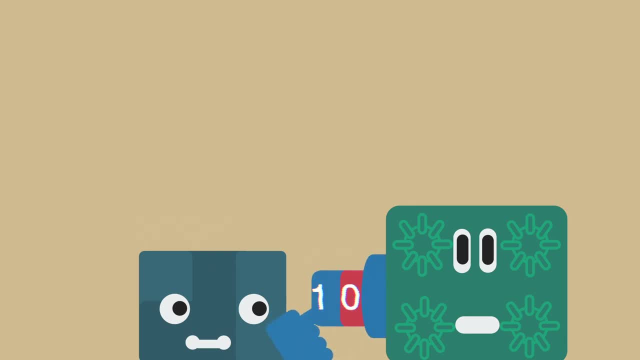 The problem is that a quantum computer only needs to ask the oracle once to answer this question, thanks to its use of superposition. In this case, we can imagine the quantum algorithm to be my friend on the right and the classical algorithm to be my friend on the left. 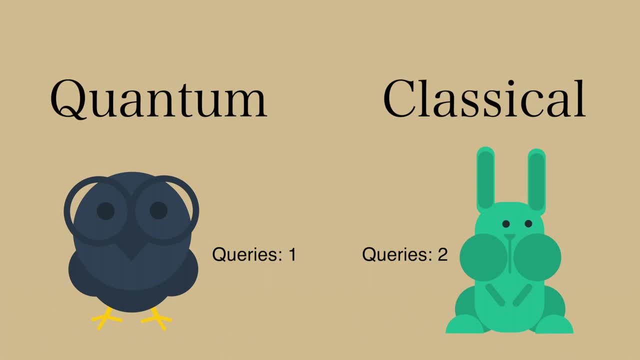 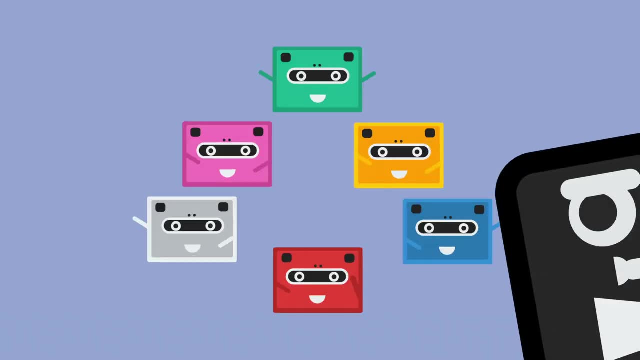 They can both solve the problem, but the quantum algorithm needs to ask the oracle fewer times. Therefore it is more efficient. Just to reiterate: this problem serves no practical purpose. None of the black box problems do, But they were the first true quantum algorithms.